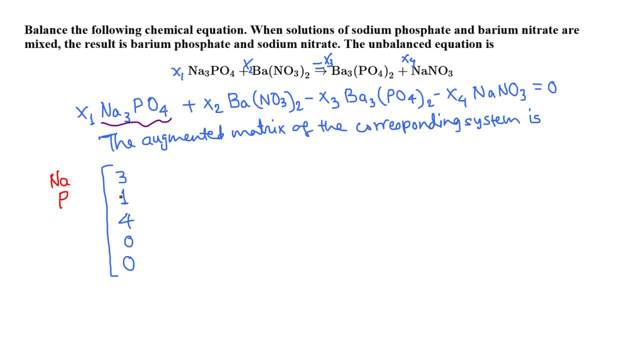 phosphorus one. So just P and oxygen 4. So oxygen, and if we look at carefully, we got barium Ba, but there there are none. so zero, zero bariums Ba. and we got N nitrogen In this first term there are no nitrogen. so 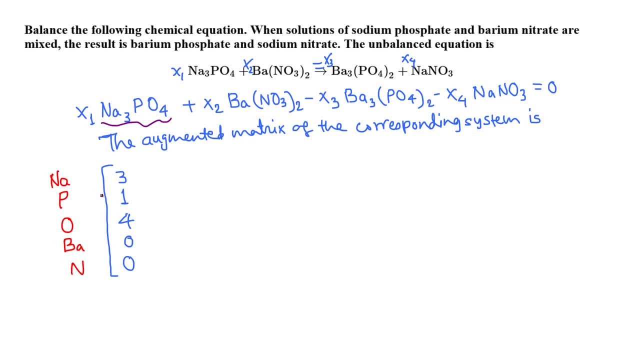 zero nitrogen. So we are writing in this way for each of these four terms. okay, So in the second term, barium. so barium, we got just one nitrogen, two of those two, oxygen: six and nothing else. sodium and phosphorus: zero. On this third term now, 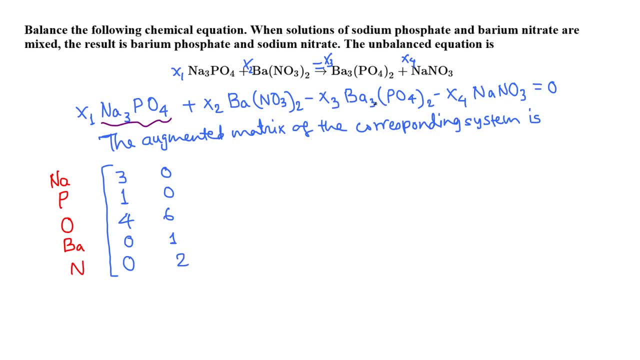 negative Ba3, so Ba3, but we got negative three because we move to the left side. barium three, P2, the phosphorus two, but negative oxygen eight, but negative eight. okay, and then no sodium, No nitrogen In this fourth term. now there's a negative sign here, by the way. 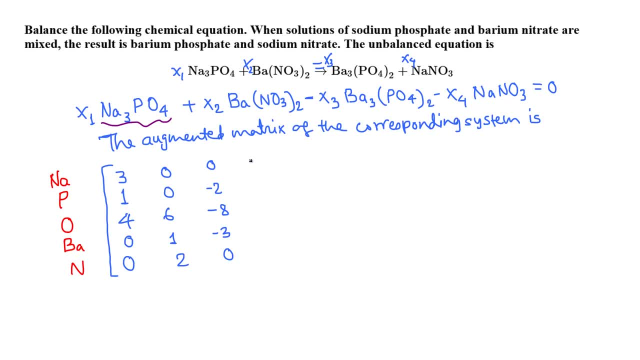 sodium, one, so Na1, but negative. one. Nitrogen, okay, just one, but negative because of this negative sign. O3, oxygen, three, that's negative. and this phosphorus, non barium, non zero, and is equal to right hand side zero mean nothing. all zero, zero, zero, zero, zero, zero. so in this way we can set up a 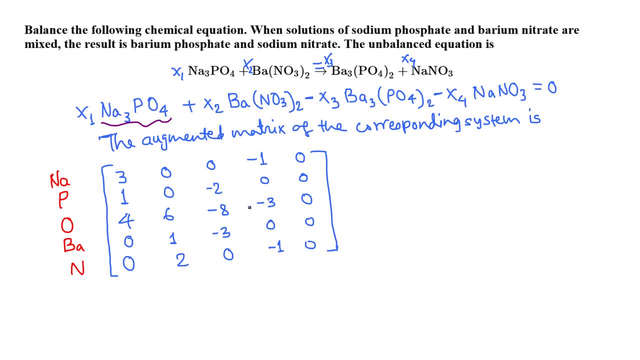 system whose augmented matrix is this: okay, now we're gonna do some row reduction and write this in row echelon form. okay, we try to make this one, if possible, the second row. so let's swap first and second rows so that we get one here and that makes our life easier. okay, so swap R1 and R2, R1 and R2. okay, so the 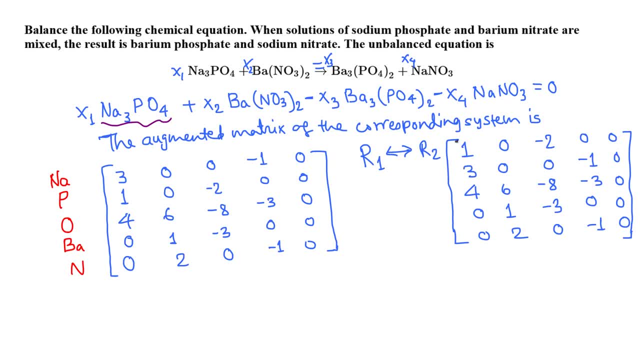 next we want to do is: this is pivot. so when I make zero here, zero, zero, zero, and we wanna put some pivot there if possible, zero, zero, zero, pivot, zero, zero, pivot, zero. okay, so we want to make this zero. look at this: this r1, r2, r3, r4. if we move up, then 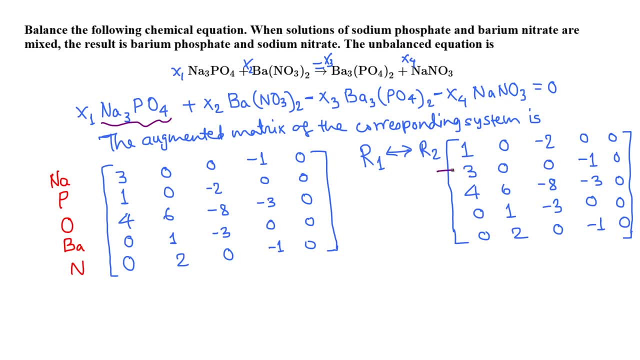 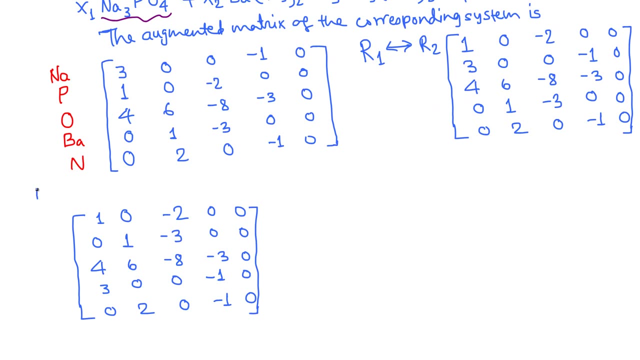 this becomes zero. okay, so we want to swap these two terms. that means we want to swap r2 and r4. so I just swapped r2 and r4. so r2 and r4, we have this. so this is good. zero one not needed, but one helps. now we're going to make this. 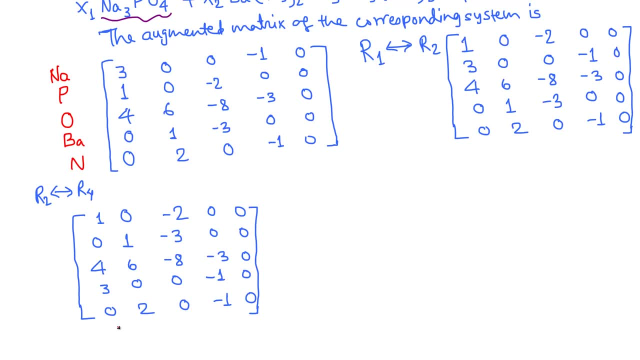 zero here. okay, here we got zero, so we can swap r3 and r5. so let me write over there. so we swapped row 3 and row 5, so we have zero here. next, we want to make this zero using this pivot one. at the same time, we can make this zero using one as well. so we want to do the. 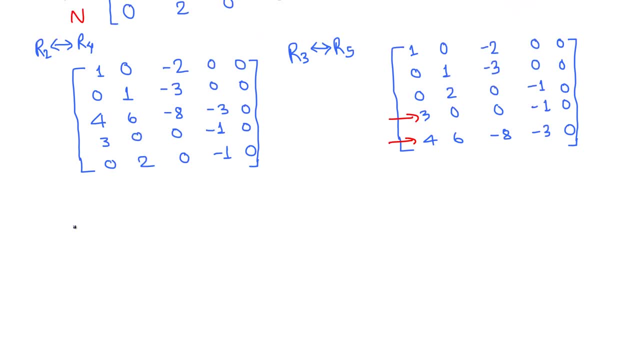 following: so we're going to work on r4 such that r4 plus negative 3 times r1 and r5, that is, r5 plus negative 4 times r1, okay, and the first three rows stay same and we do this. so with these operations we are here. next one: all 0 is good. here is a pivot, so you want to make. 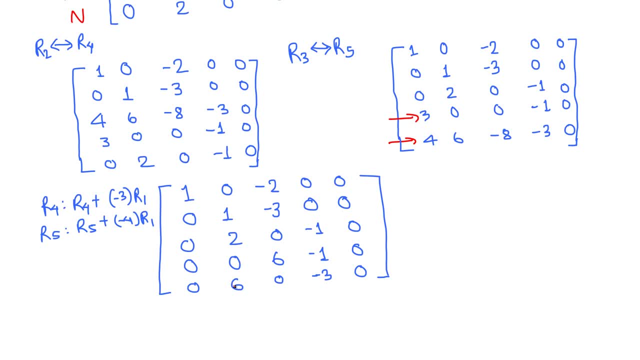 this: 0, zero, zero, so one, and now there should be non-zero, if possible pivot, and then zero, zero and non zero and zero. okay, non-zero means pivot. sometimes, if we, if we find one row multiple of another, then we can make the bottom row zero, because we can subtract by suitable. 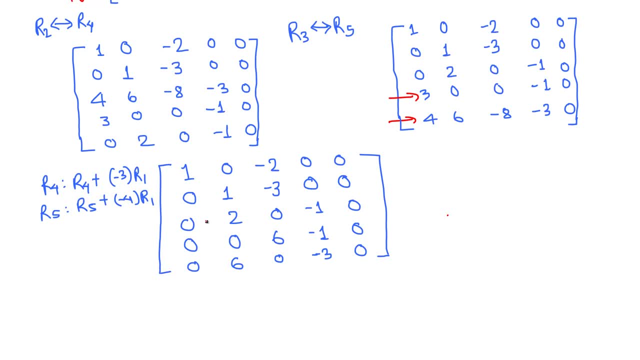 multiplication and it becomes zero. Looking at these two, look at r3 and r5- two goes three times. if we multiply this by three, three times two is six, three times negative. one is negative three. so pretty much this one is three times this. so if 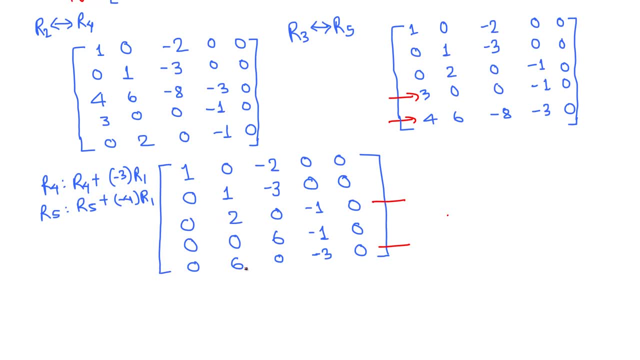 we multiply this by negative three and combine with this, we're gonna get all zeros. so I'm gonna change this to zero, zero. I mean, this is the case all the time when two rows are just multiples of one another, then we can just make all. 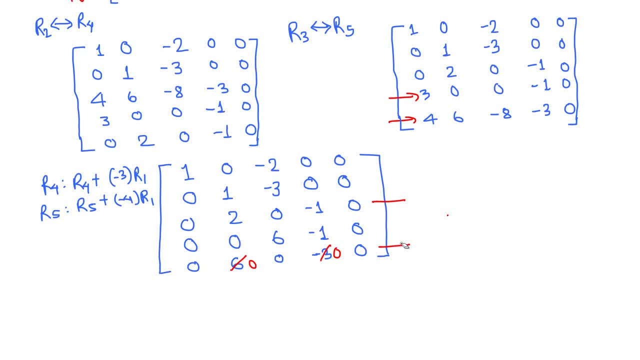 zero. this is good enough. so, and we always write all zeros on the bottom row. okay, that's good. Now next, we still want to make this zero. okay, to make this zero. look at here: zero. if we swap, then will be good. so that's r3. 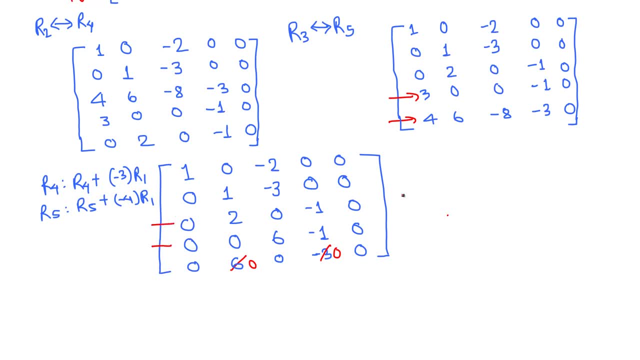 and this is r4, so we just interchange r3 and r4. okay, so we swapped r3 and r4. we are in this place. okay, we should have made this zero now. same thing: now we need to make this zero. Okay, for this, we use this pivot. so, using r2, we want to make this zero. so org on r4. 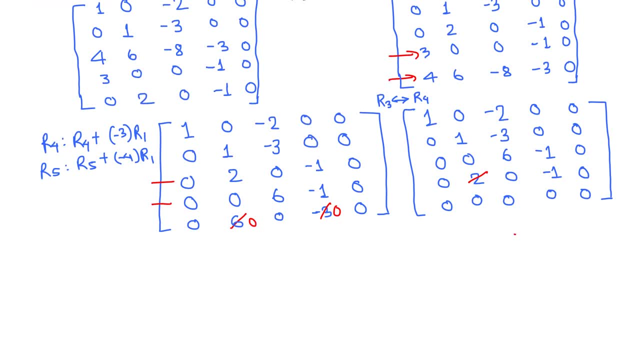 okay, so org on r4 using the pivot, this one. so this will be r4 plus negative 2 times r2. multiply this by negative 2, and 2 plus negative 2 is 0. so we do this and when we move all zeros. 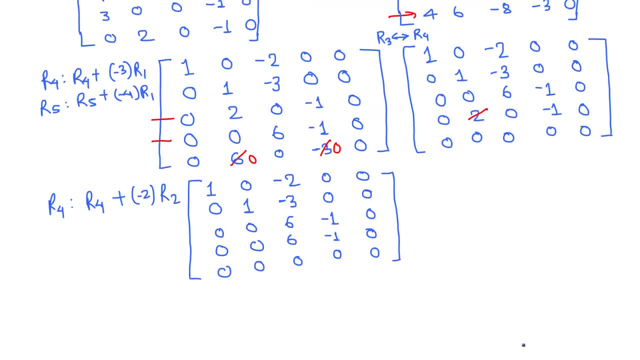 On the bottom row. okay, let's do so performing this operation: r4 plus negative. 2 times r2. this is r2 and r4. 2 times negative. 2, 0, 0 times positive. 6 is 6. negative, 1 times 0 plus there is 0.. Oh, we got now r3 and r4- the same. look at: 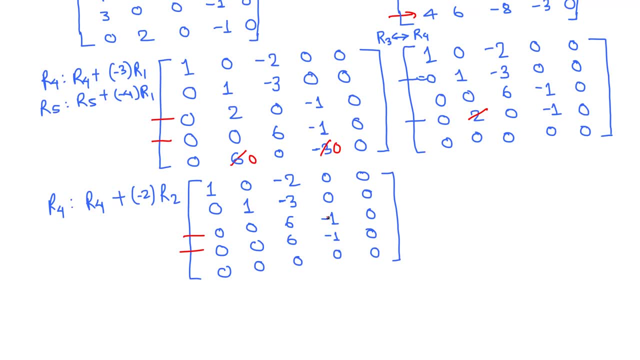 these two rows. they are same. that means we can just multiply these two rows and this by negative 1 and add with this, so we can make all zeros. so basically we got two zeros, two rows of 0. okay, so let me write that. so we are getting this. 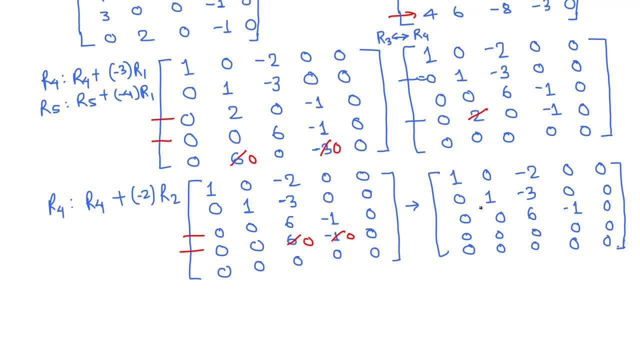 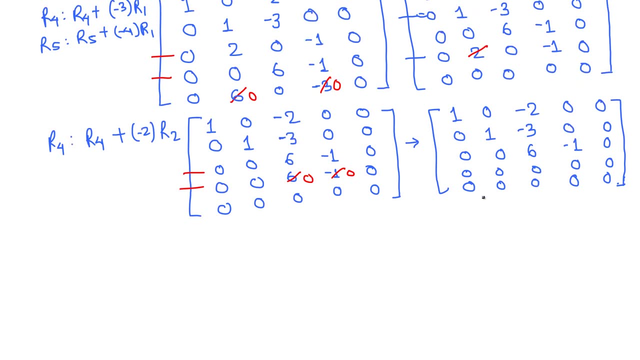 matrix. okay. so this is x1, x2, x3, x4. now this is in row is learned form and we can solve for x1, x2, x3 and x4.. So this is x1, x2, x3, x4. now this is in row is learned form and we can solve for x1, x2, x3 and x4.. 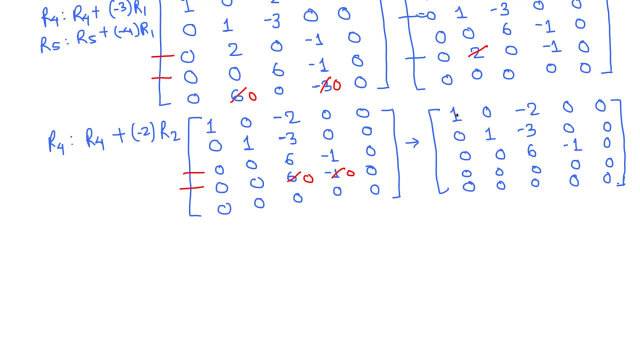 Looking at this. so we got this pivot here, we got pivot here. we got pivot here. there is no pivot, so this is free variable, so that is x4 and we don't have pivot in the last column. that means good, we have a solution, in fact. in fact there. 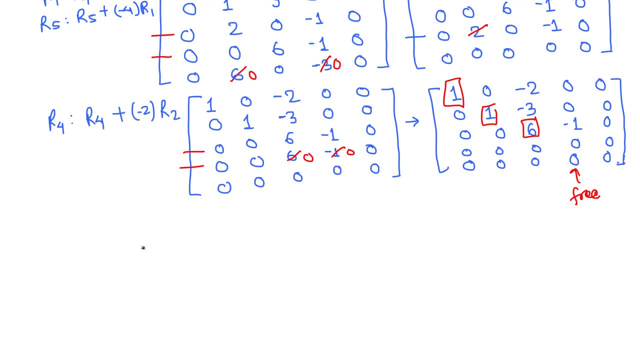 is a free variable, so we have infinitely many solutions. so free is the fourth. so this implies x1, x2, x3, x4 and x4.. So this implies the fourth is free, so we can choose anything of our choice. going back to this third row, that's the 6x3 minus x4 is 0. okay, now we add x4 to the. 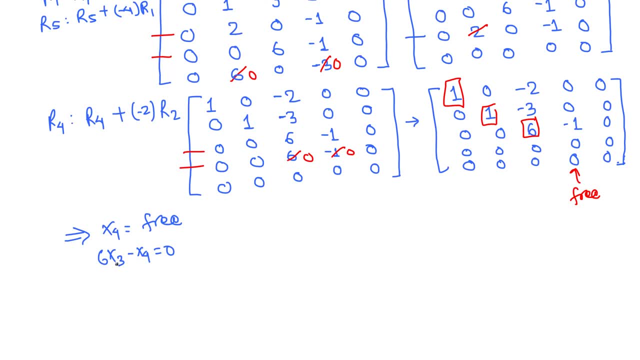 both sides and x4 is free. just keep x4 divided by 6. this implies x3 is 1: 6th x4.. So this implies x3 is 1: 6th x4.. So this implies x3 is 1: 6th x4. 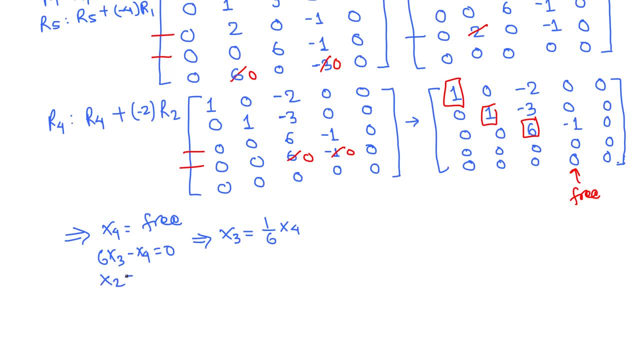 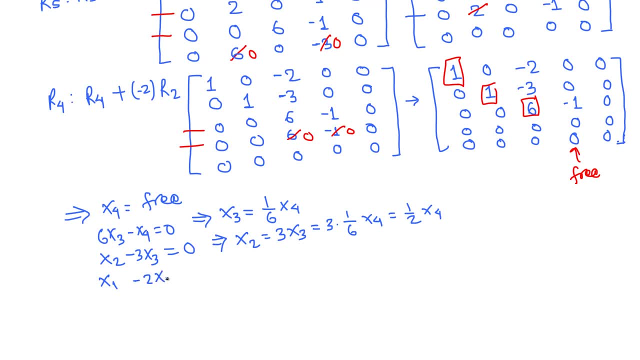 minus 2x3, because the x2, second row, nothing equals 0. that implies x1 is 2x3 and x3 is 1 6th of x4. so this is 2 times 1 6th of x4. so that's 1 3rd of x4. so we 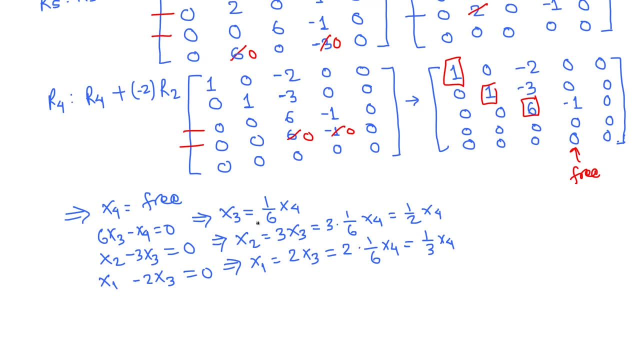 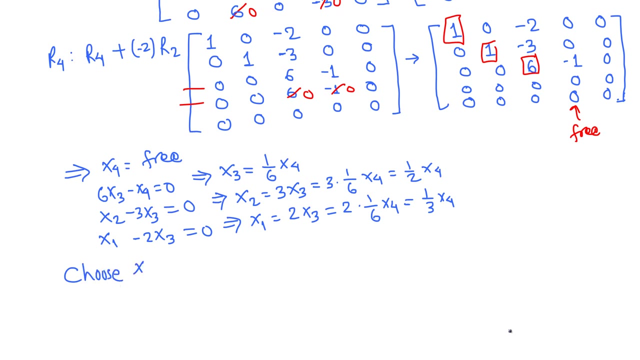 are looking for just one solution. in fact, if we keep x4 as a free variable, we have infinitely many, but we just want to balance the chemical equation. so let's choose x4 to be any real number of our choice. so we want to choose x4, so 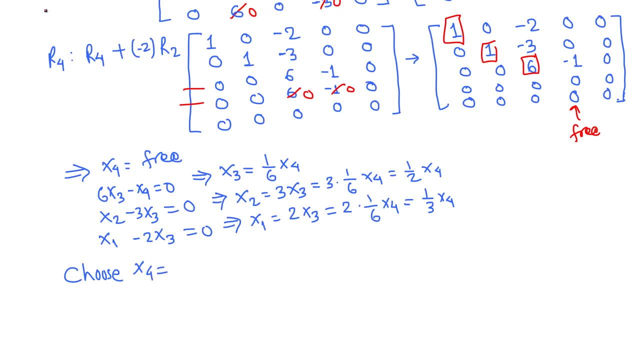 that we don't get these fractions. okay, we have. this is free anything. look at here: 1, sixth, so x4. if we choose like 6 or 12 or 18, then 6 divides. at the same time, that number should be divisible by 2 and divisible by 3, oh 6 is divisible. 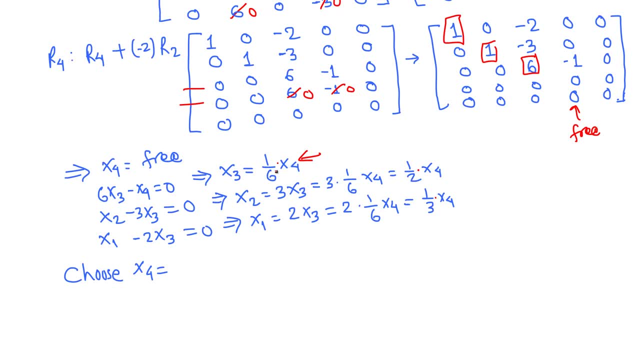 by 2, divisible by 3 and also by 6. we can just choose x4 to be 6, then we can write everything now. then this is x 1. by the way, x 1 is one-third of 6. That is 2.. X2 is 1 half. 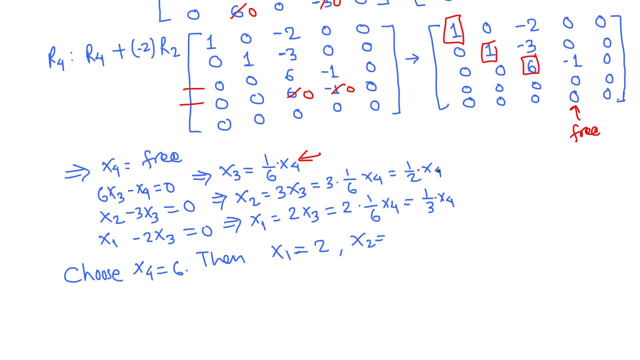 of 6,~. but at least 3 is divisible. so it is divisible by a 2, so divided by 3 is редguised. So this didn't get really easy. so you made a really simple things. we can just x4, 1, half of 6,, 3, x3 is 1, sixth of 6, just 1, and x4 we just chose 6.. So we're. 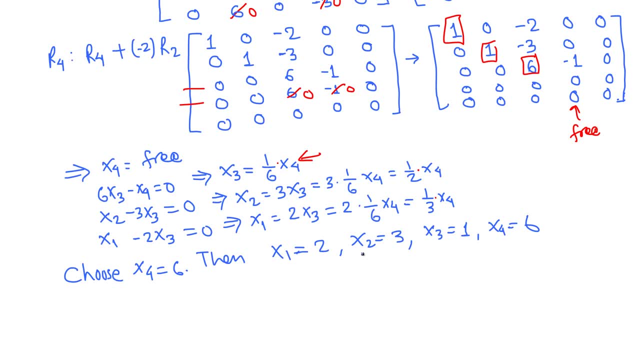 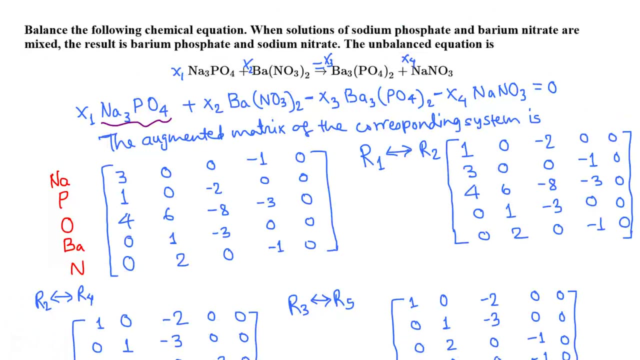 going to plug this back on the top 2, 3, 1, 6,, 2 3, 1, 6.. So come back here, so the equation will be so here. I want to write this balanced equation in this way, so we: 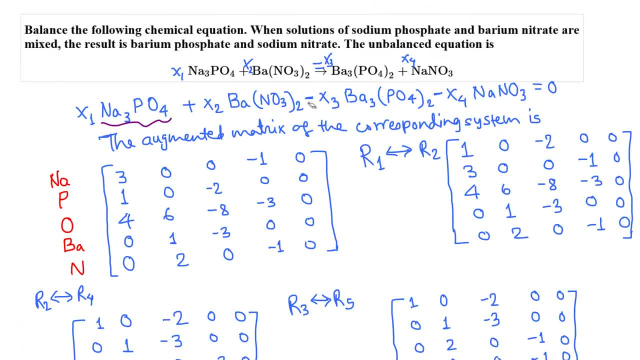 know x1, x2,, x3, x4, so if I move to the right side, I'm gonna get equality sign here. okay, I'm gonna get equality here and this will be positive. in fact, there is no equal. when we move, then this will be plus. So what are the values of?